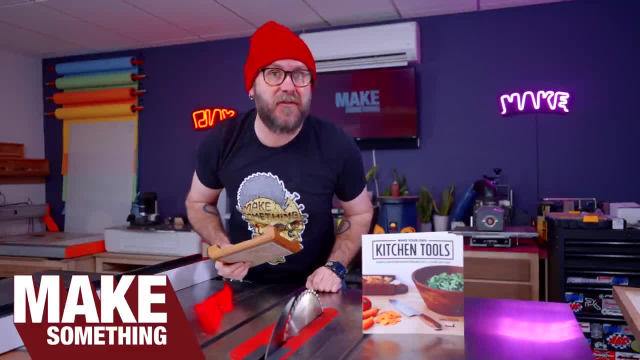 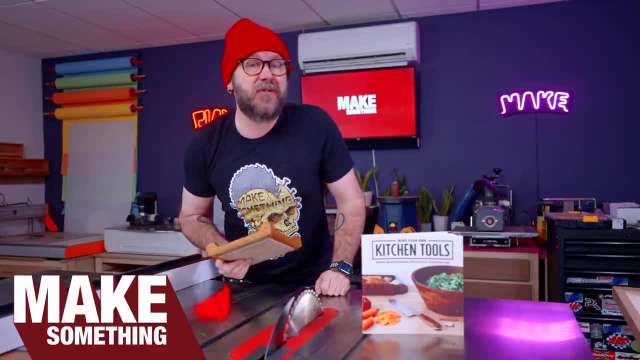 This is not your grandfather's trivet. It's actually my grandfather's trivet. He's made a bunch of them. He gifted me this one and I liked it so much that I put it in my book: Make Your Own Damn Kitchen Tools. Today we're going to 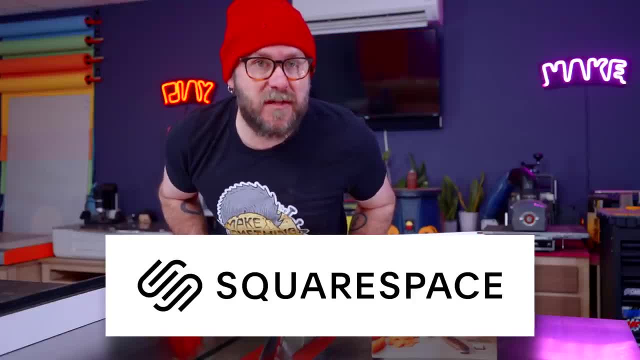 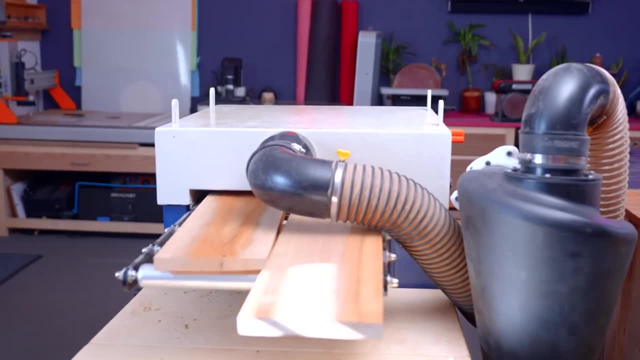 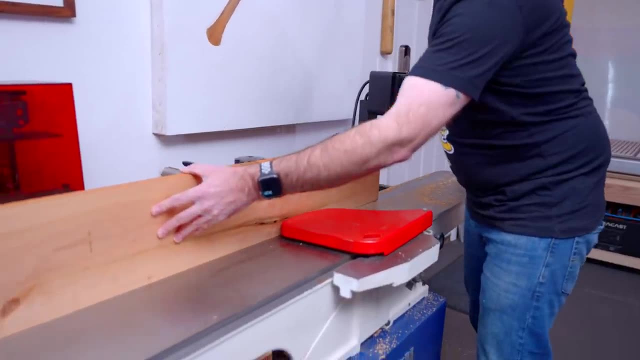 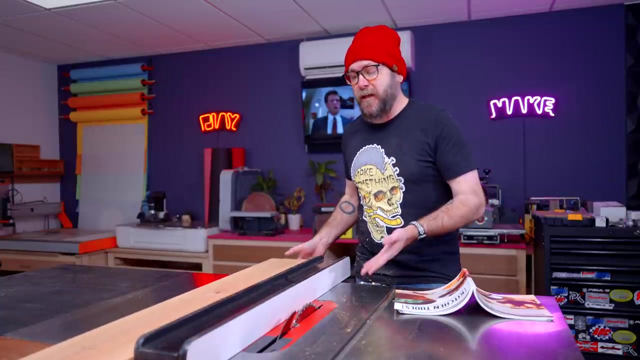 make a bunch and give them away. Today's video is brought to us by Squarespace. This is some locally grown cherry that comes from my grandfather's friend, So thank you, Al. It does come rough, So I had to mill it up, and now I'm here at the table saw. 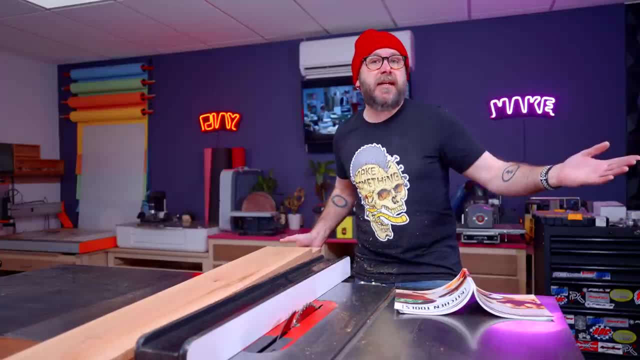 There are some defects that I got to work around. I don't know how many I'm going to get. I'm just going to go with the flow today. If we get one, we get one, If I'm able to get four. 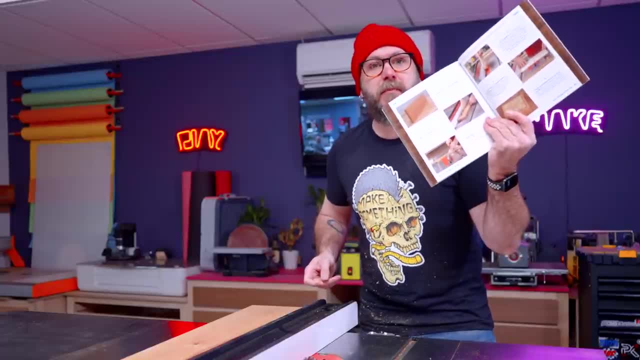 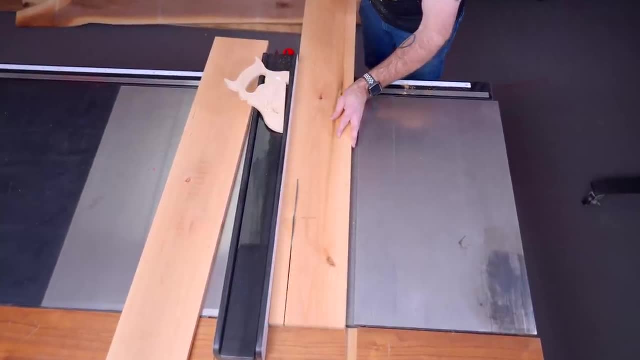 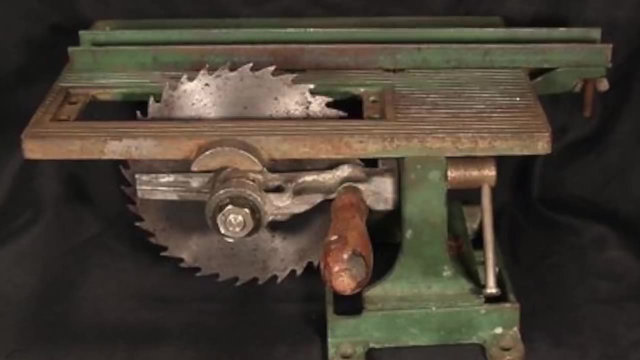 five. we get four or five. I'm just following the steps here in my book. and step two says I need to cut one and a quarter inch strips here at the table saw. Don't be thinking you need a big fancy table saw to do this. You can use a contractor saw that you get from your local Kmart. 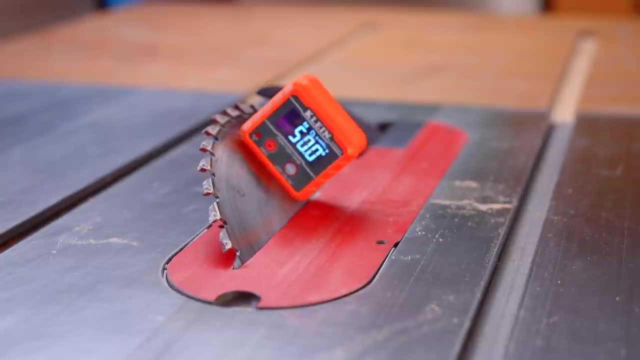 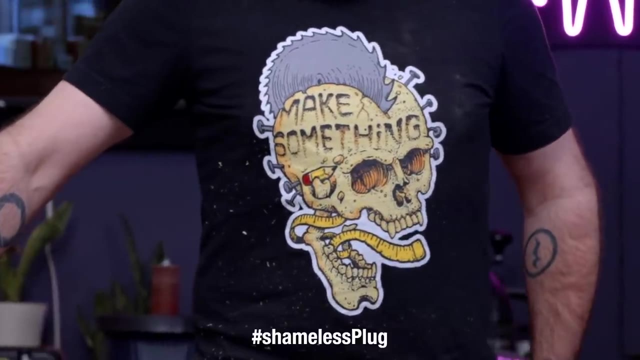 Now I'm just setting my blade to 45 degrees. It's 12 degrees outside and I'm wearing a t-shirt. What's up with that? I have my blade set to 45 degrees. It's time to cut all of these to length. 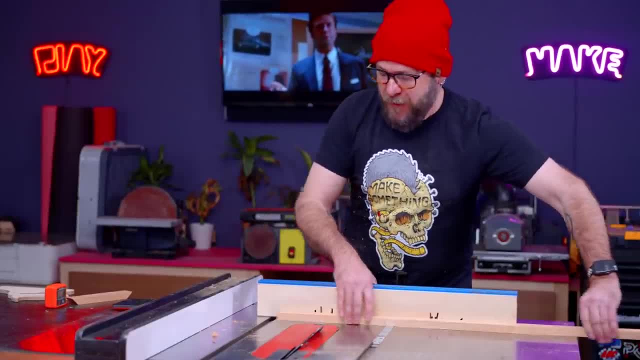 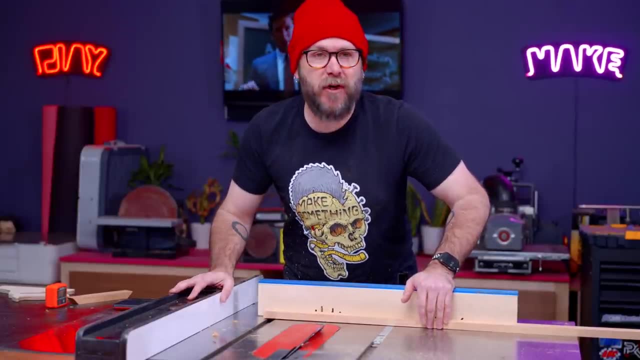 So I'm going to run them through, flip it over and then run it through again to cut that length. You never want to use your miter gauge and your fence at the same time. It will kill you, So I'm going to use my fence and a spacer to get all of them. 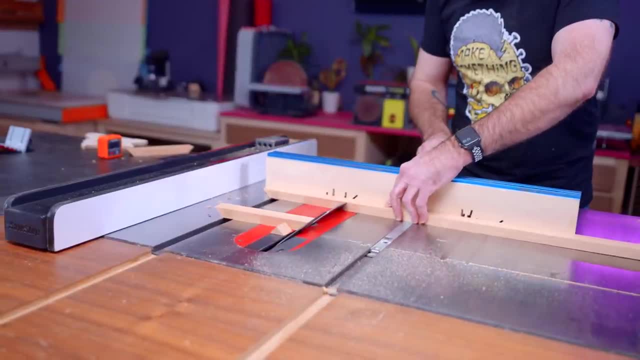 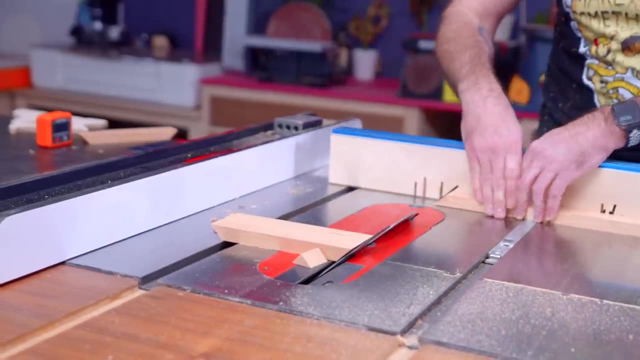 to that perfect length. I'll pull the spacer out and then run this through. A couple of hot tips for you. You want to push the pieces past the blade. That way, when you're cutting the next piece, the previous piece doesn't vibrate. 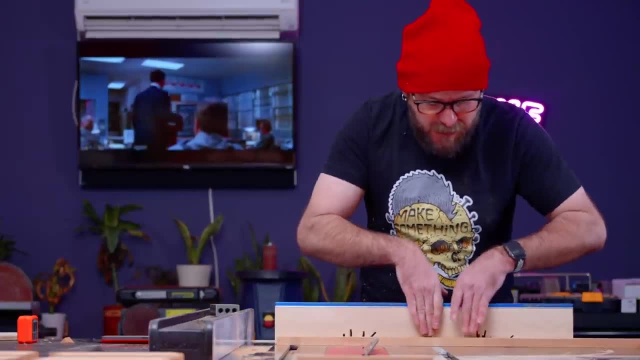 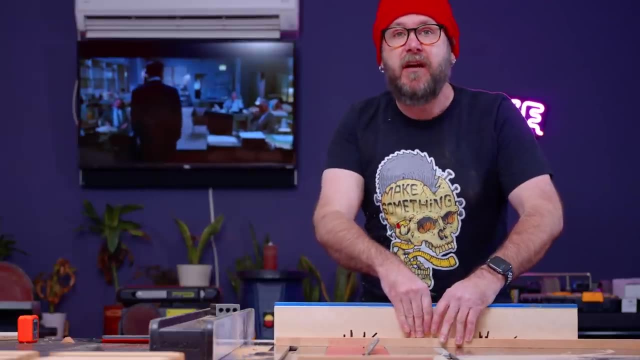 hit the blade and then take out your face And also some of these boards. there's a little springiness to them. They're not laying completely flat on the table. You want to make sure you're holding them down flat, Otherwise you're not going to get a perfect 45 degree angle, and it's going to be. 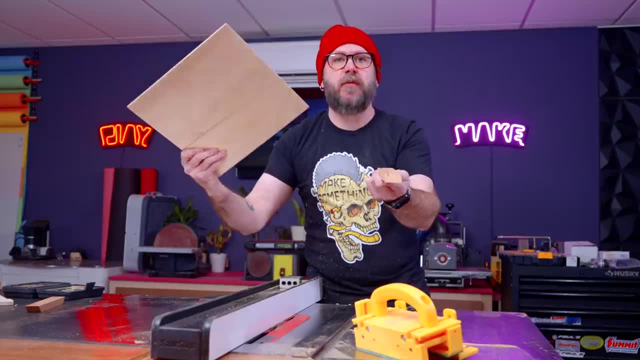 a couple of degrees off. Next up, I'm going to be cutting a little bit of wood here. I'm going to be cutting a little bit of wood here. I'm going to be cutting a little bit of wood here. Next up is to cut a groove to hold a plywood bottom. 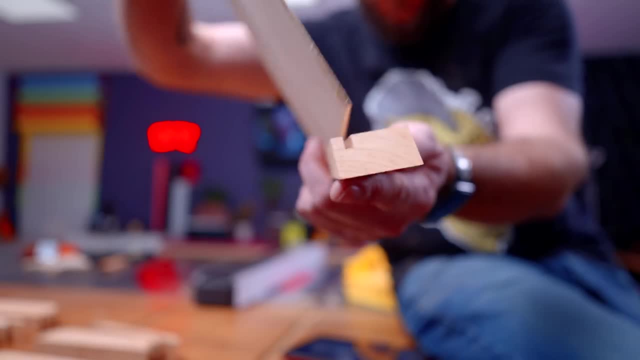 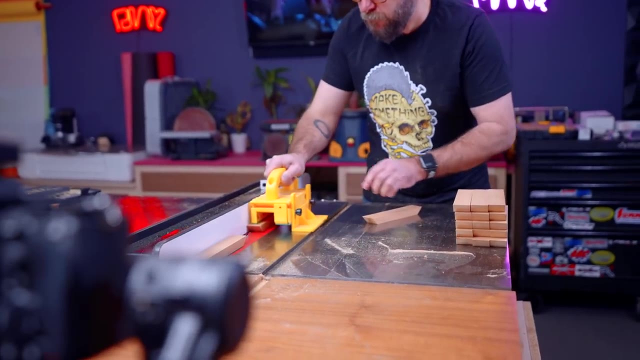 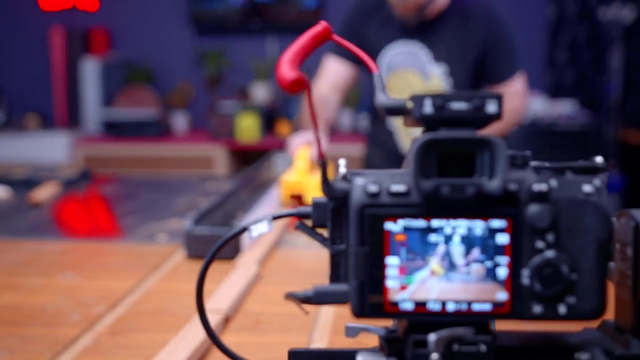 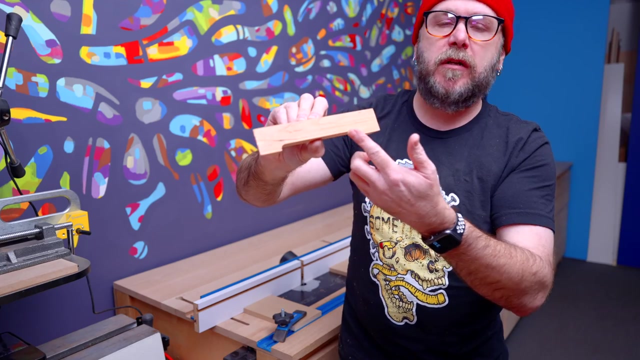 I'm using 1 1⁄8 inch plywood, So the blade is the perfect width for that. Unless you're using a thin curve blade, then you might need to make a couple of passes. Now I'm going to cut this groove along the bottom. 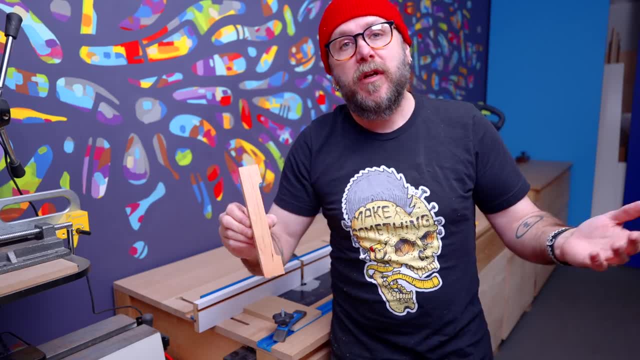 That's going to make it look like it has feet. That's going to make it look like it has legs on the corners in the book. We do this on the bandsaw. today I'm going to do it on my least favorite tool. 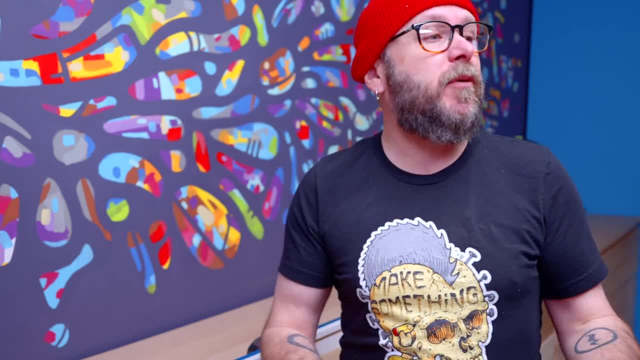 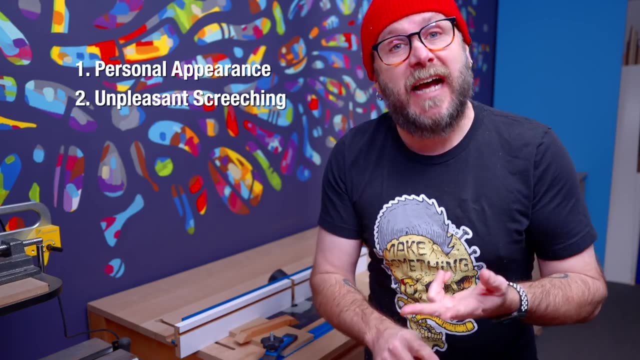 I thought it was obvious why the router was my least favorite tool. but people keep asking me, David, why is the router your least favorite tool? I don't like the way it looks, I don't like the way it sounds, I don't like the way it makes dust. 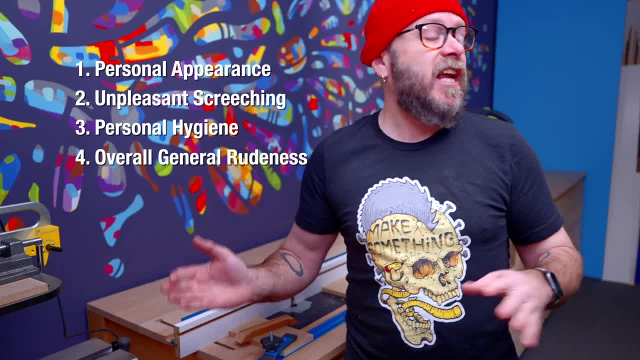 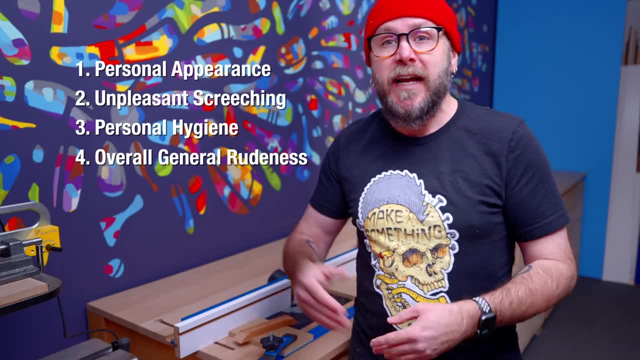 I don't like the way it'll take off your fingers and you won't even know it. If you cut off your fingers at the table saw, they'll at least be laying there so you can see that your fingers have been cut off If you do it at the router. 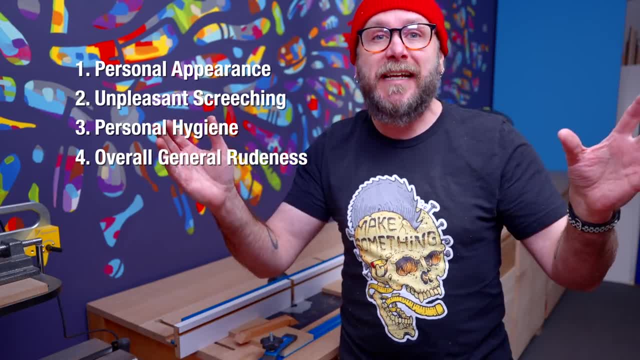 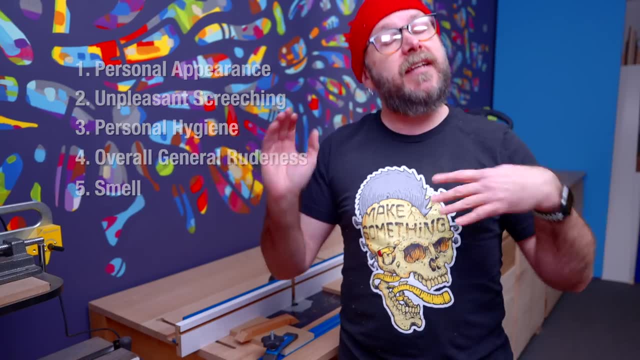 it just knurls them up and then the dust collection sucks up all the pieces and you might walk around for like 10 minutes not knowing that your fingers are gone. I don't like the router, but today I'm going to push through my hatred and I'm going to use the 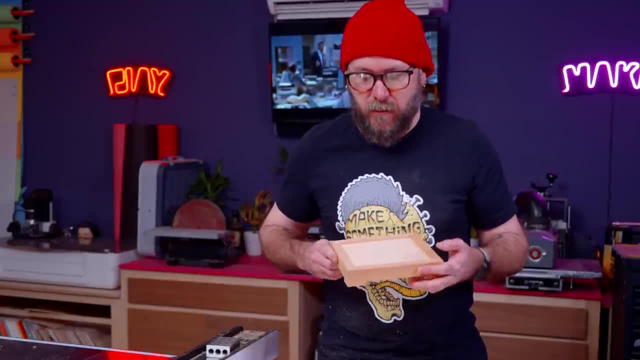 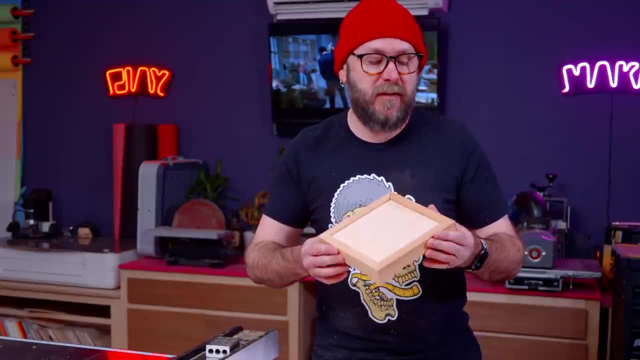 Next up. we're going to cut the plywood. that's going to fit, So we're going to go into the groove right there. You have to cut this to fit because if you cut it too big you're not going to have a successful glue up. a little too small is not a big. 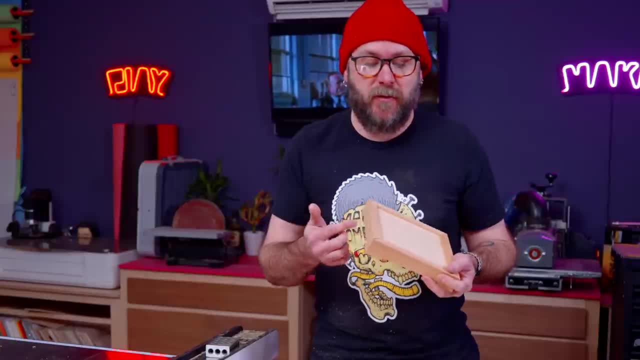 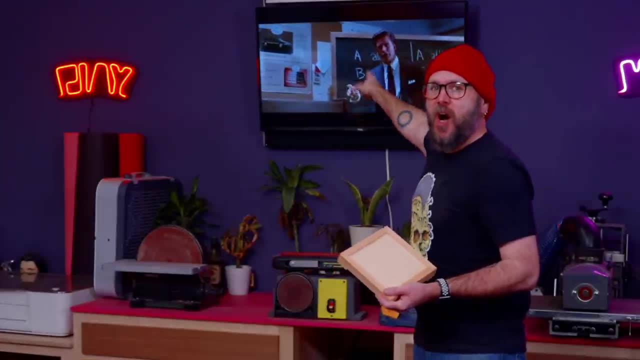 deal And we're going to glue in this plywood piece and that's going to reinforce those corners, So we won't have to do any extra reinforcements in the joints A, always, B, B, C, closing, always be closing, always be closing. 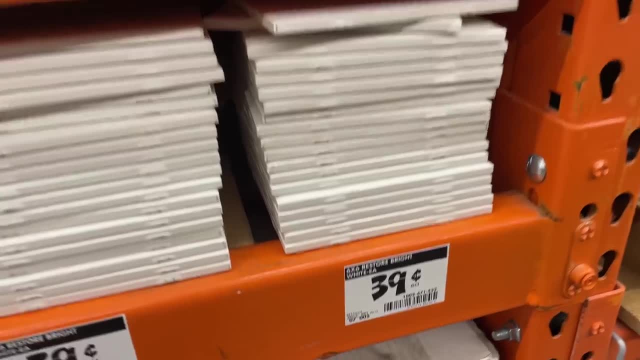 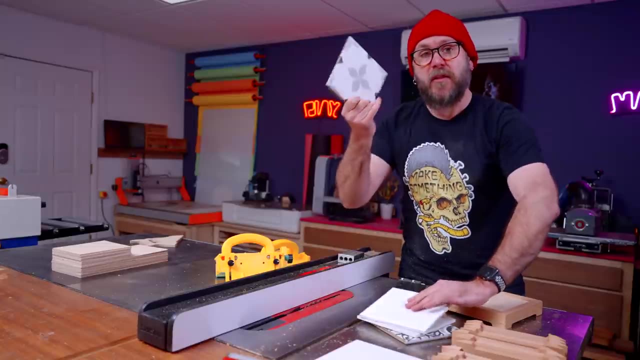 For the top we're going to use tiles that you can get from the home center. This one was like 39 cents and then this one with the pattern was like a dollar 39, somewhere around there. So this one with the pattern here that fits in perfect. 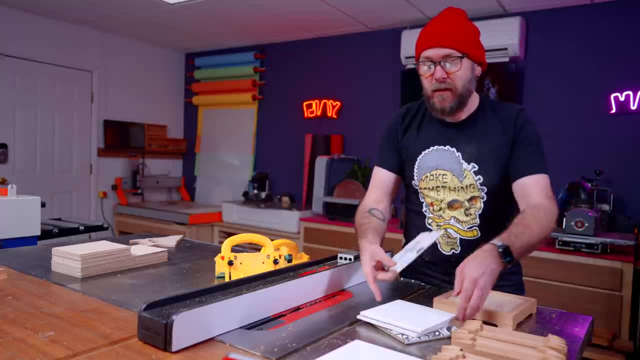 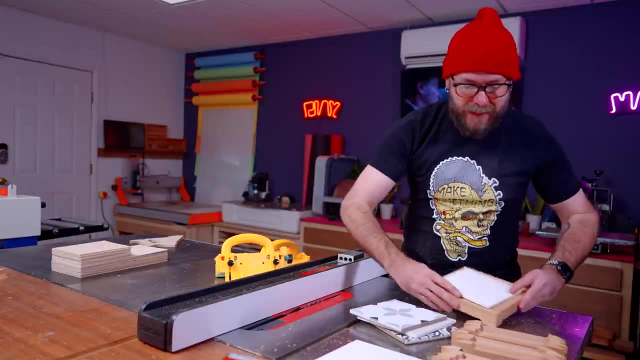 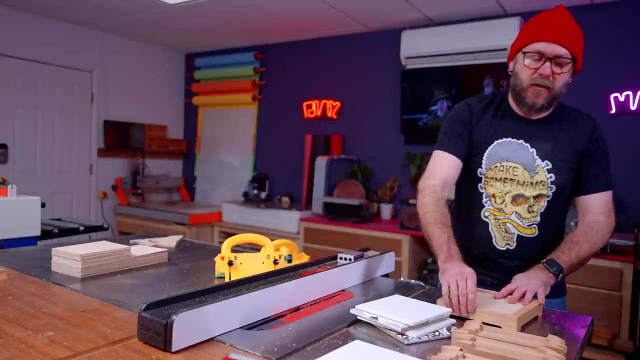 no modifications needed, but apparently not all six inch tiles are made equal, And then this white one is slightly too big and doesn't drop in there. I don't know who's in charge of the tile industry, but maybe we can work on our quality control a little bit. So what we need to do: 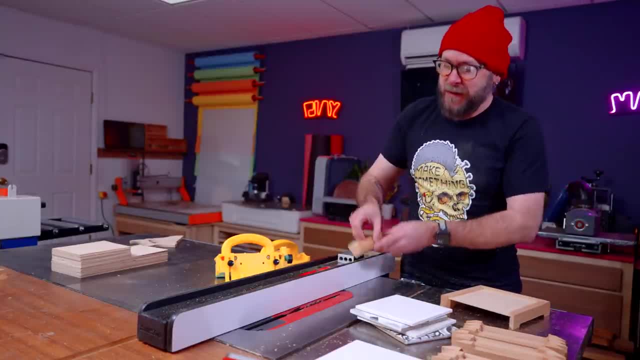 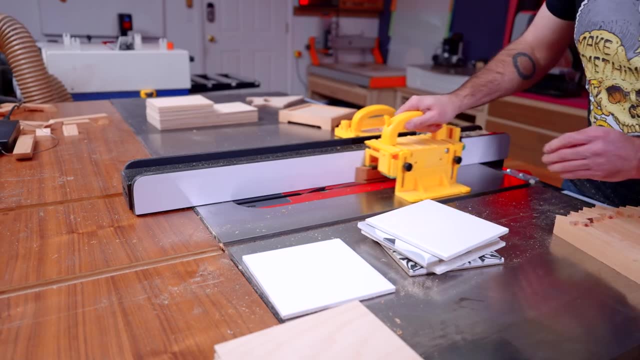 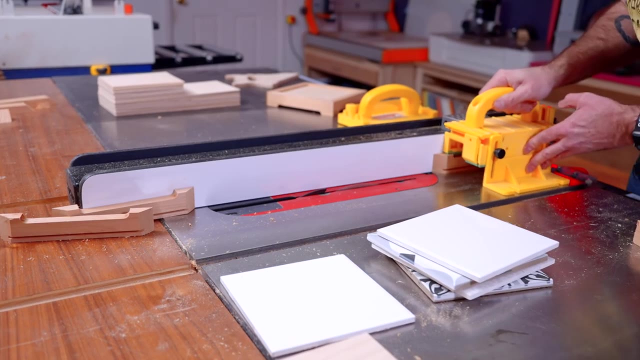 is just take off a sliver of wood on each of the four pieces. So I've got my blade just above the table and I'm going to run all four pieces along there and see if that white one drops in. Took off maybe a 16th right there. 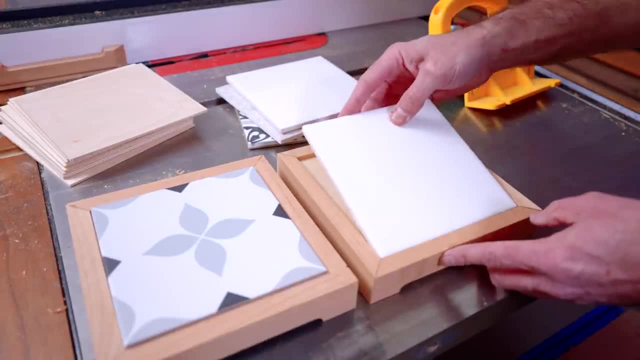 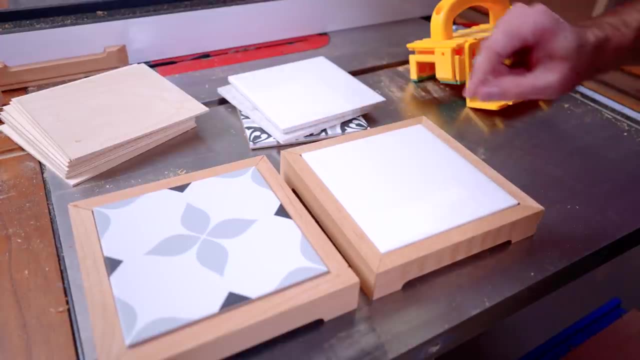 Got that rough assembled and I can drop this in to see if it fits and that works. So anything with the super cheap white tiles, it has to be cut slightly bigger. So now let's go glue this up. I went ahead and drilled a hole in the center of all the plywood bottoms. 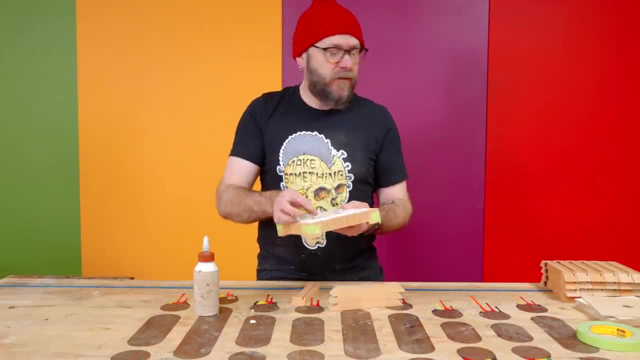 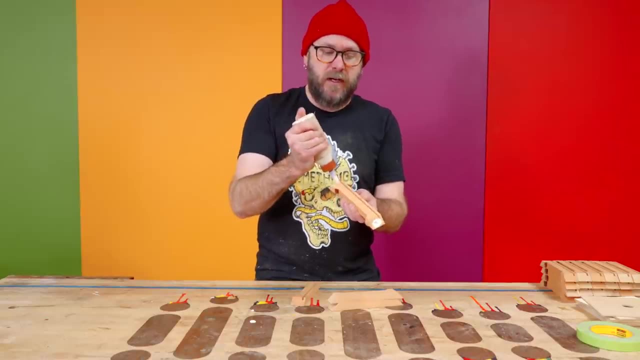 That way, you have a place to put your finger to remove the tile if you need to. So now I am gluing this up, And while I am gluing this up, I would like to tell you about today's sponsor, And that is Squarespace. 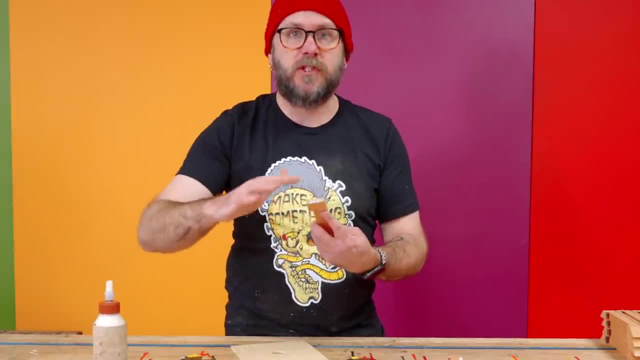 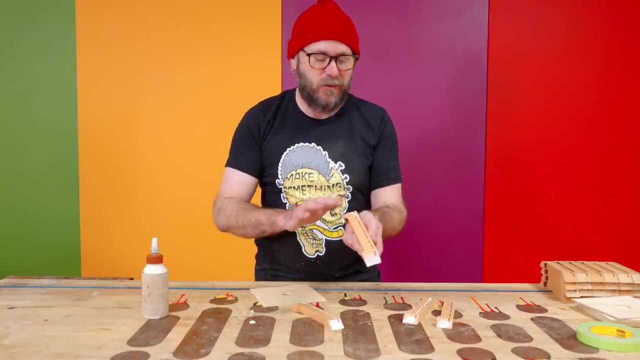 If you are like me and you like making things, which I hope, so I hope that's why you're watching this video- You need a website. You already know why you need a website. You need a website cause it's 2022 and you need a place to show off your work. 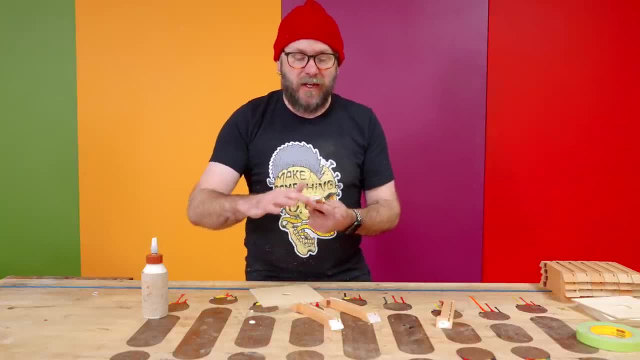 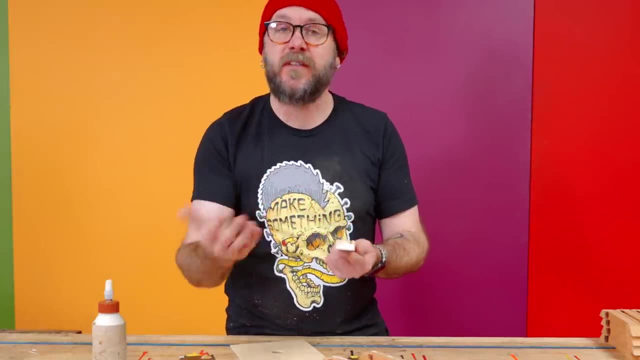 You need a place to get clients. Maybe you want to sell some of your crafts. Maybe you're really good at designing crafts and you want to sell plans for those. You could do that on your Squarespace site. You can sell both physical and digital items. 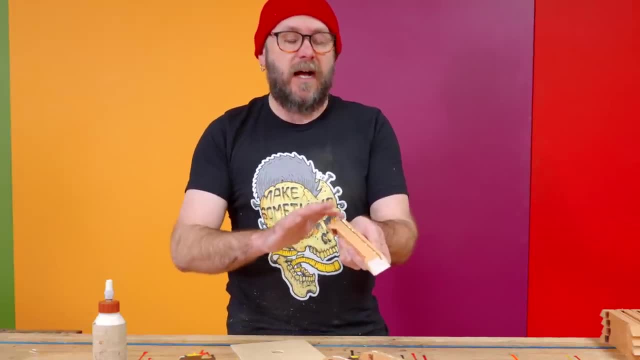 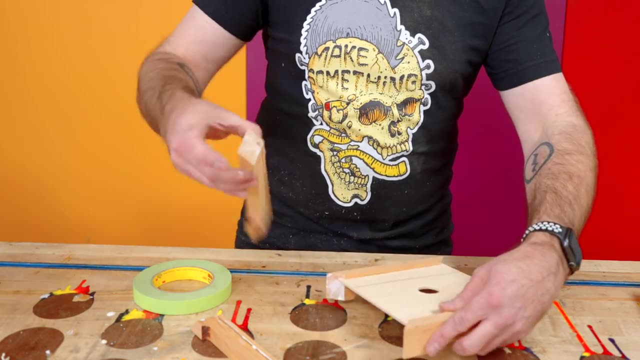 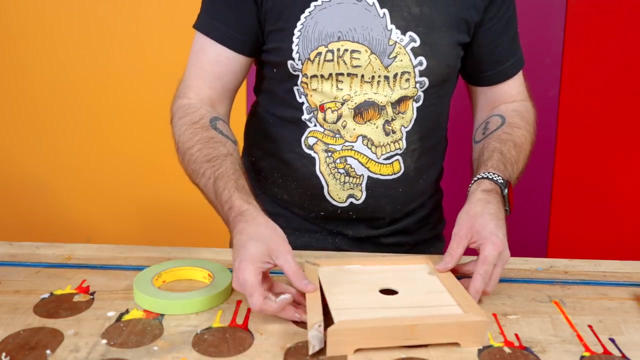 If you went to my website right now, you would see that I sell both digital and physical items, as well as merch and all kinds of stuff. I've been using Squarespace for a long long time, long before they were were a sponsor- and the reason for that: it is super easy to use. 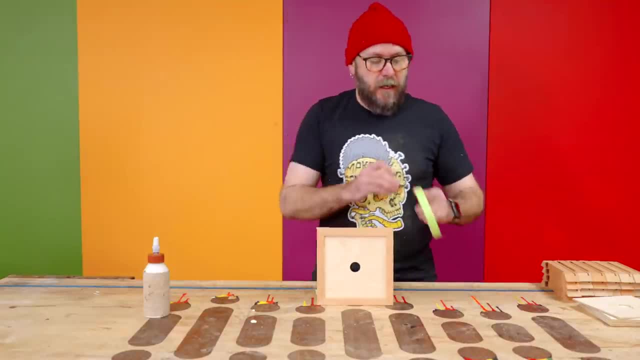 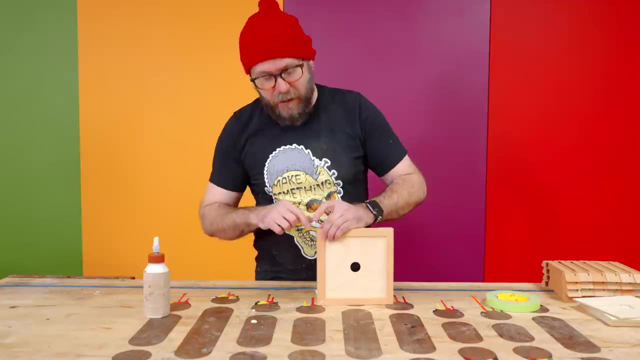 Like I mentioned before, I used to be a web developer and I got tired of making websites. I wanted to make things with my hands, So I moved over into woodworking and now I make these woodworking videos and I no longer have to deal with the cloud, the backend. 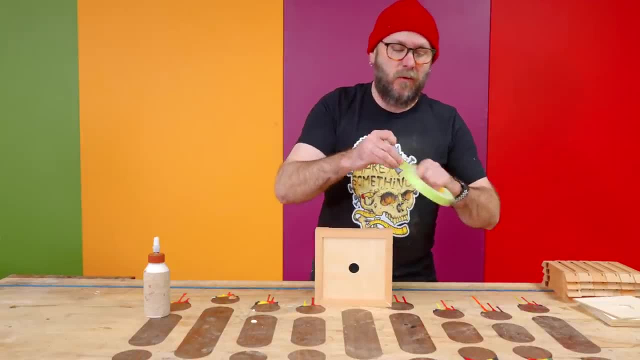 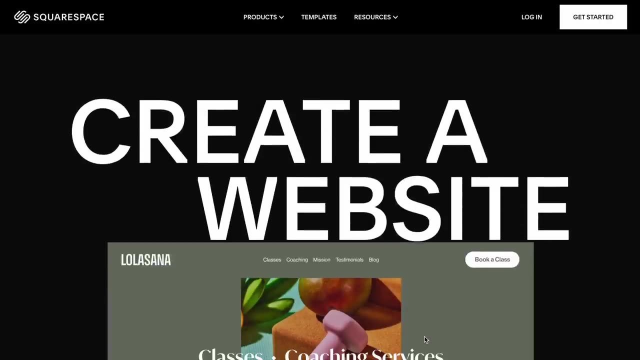 all that stuff that you got to deal with when making a website. Remember how I mentioned. if you are like me and you make things and you want to sell those things, as a thank you to those of you who stick around and support my sponsors and who